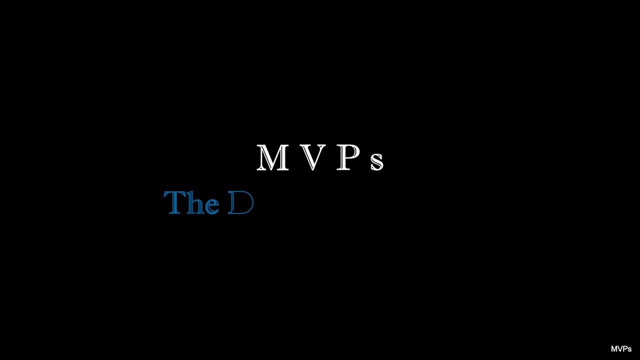 Let d and n both be positive integers. This means that we can arrange d dots in a line and we can arrange n dots in a line. The theorem we're interested in says there exist unique integers- q and r- with zero less than or equal to r less than d. satisfying the equality n equals q. 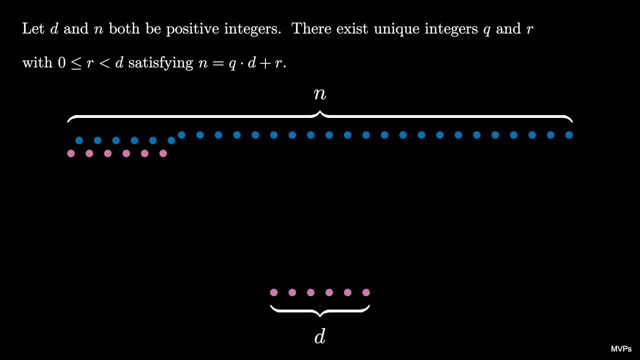 times d plus r To prove the existence of q and r, we start subtracting copies of d from n. As we do this, we create a list of decreasing positive integers By the least integer principle of positive integers. we know that this set must have a least element, as we see here, where we can no. 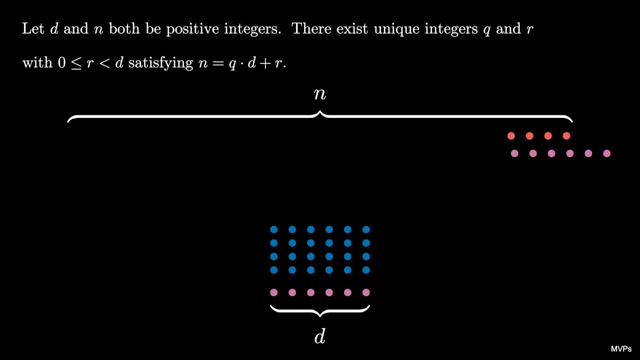 longer subtract off d. This is going to be the value of r. As we see in the diagram, we have arranged the n dots into a d by q array, with r dots left over in a line on top. This means that n equals q times d, plus a remainder of r To prove the uniqueness of the pair q and r. 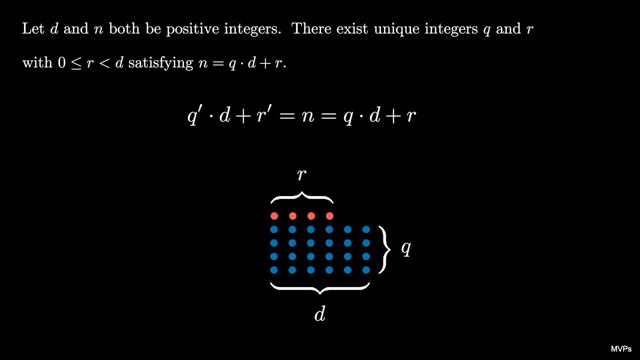 let's imagine that we have another pair, q prime, r prime, satisfying the same conditions. Because these two are equal, we can subtract to see that q prime times d minus q times d is equal to r minus r prime. But now, because r and r prime are, 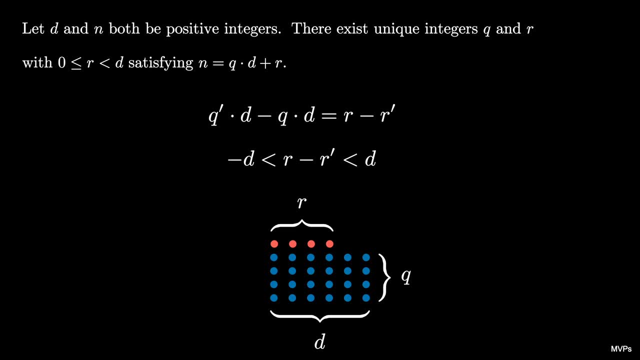 both between zero and d. their difference is between negative d and d. This means that q prime times d minus q times d is a multiple of d that lives between minus d and d. From this we see that q prime times d minus q times d must be zero, and consequently that means: 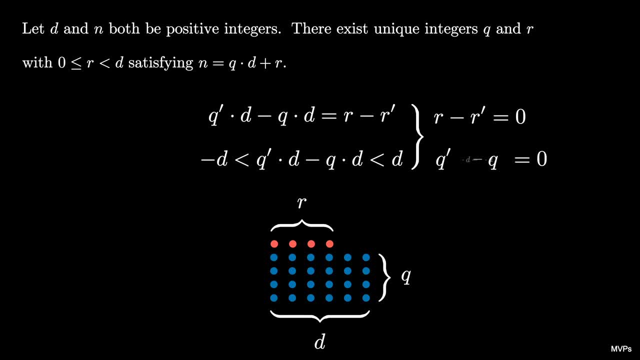 r minus r prime must be zero. Dividing this second equality by d, which is non-zero, shows us that q prime minus q is zero and r minus r prime is zero. Therefore, r must be equal to r prime and q must be equal to q prime. This means that r and q are unique. 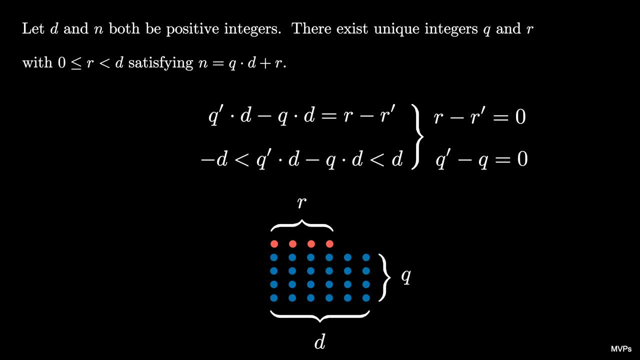 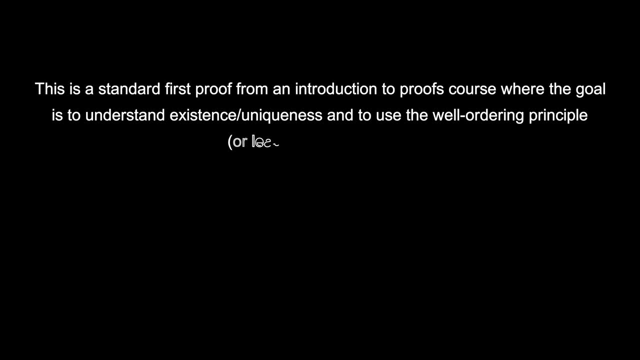 This concludes our proof of the theorem known as the division theorem or the division algorithm. Thank you very much for watching and we'll see you in the next video.